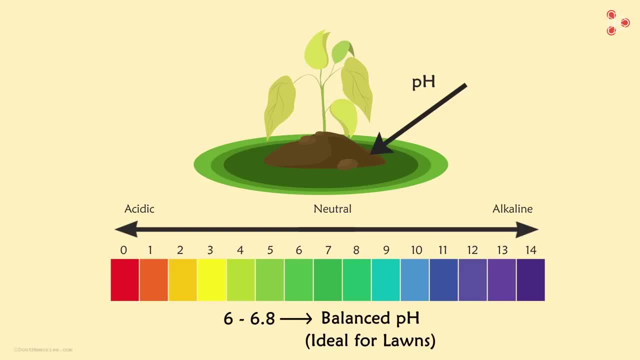 Plants cannot grow if the soil is too alkaline or too acidic. So if the soil is too acidic, its pH can be raised by adding lime, which neutralizes the excess acid in the soil. 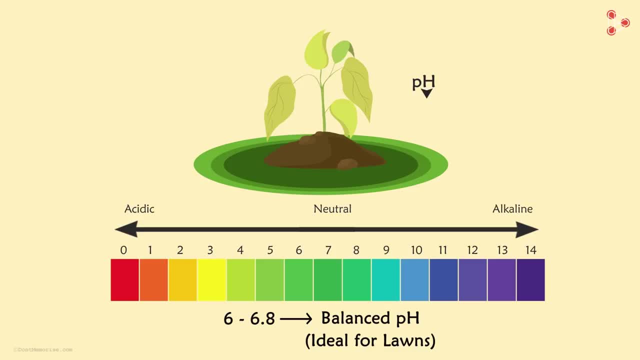 Similarly, if the soil is too alkaline, then its pH can be lowered by adding gypsum or some other substance, which can neutralize the excess alkali present in the soil. And does it affect us too? 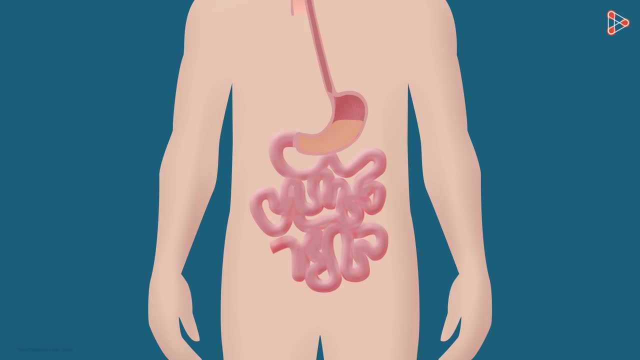 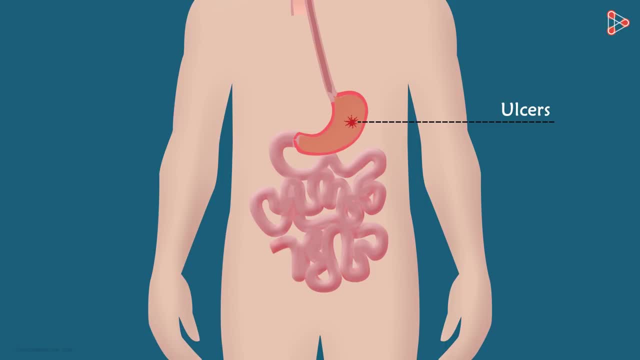 It can cause ulcers. In order to treat this hyper-acidity, a patient is advised to take antacid tablets or antacid suspensions. 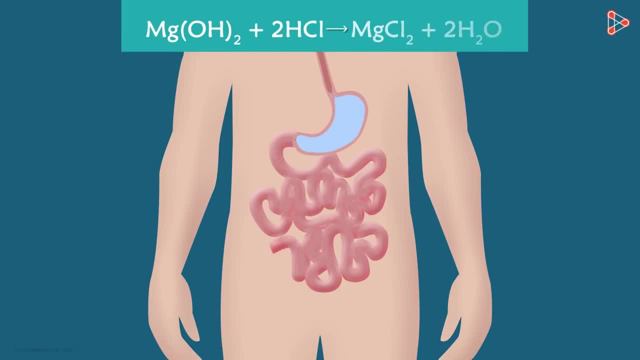 And these antacids neutralize the excess acid. 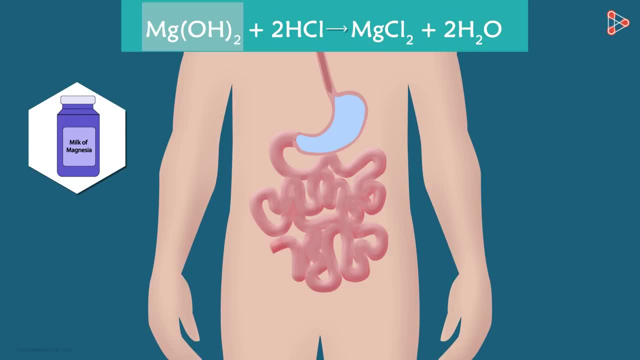 Magnesium hydroxide, a mild base, is often used for this purpose. And the reaction looks something like this. The acid is neutralized to get salt and water. 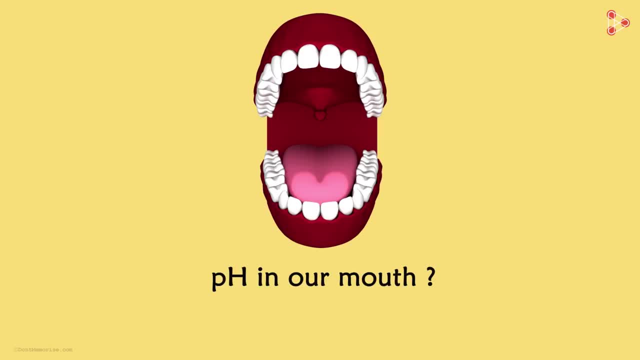 What about the pH in our mouth? Yes, the pH in our mouth? Yes, the pH in our mouth also has an effect on our teeth. 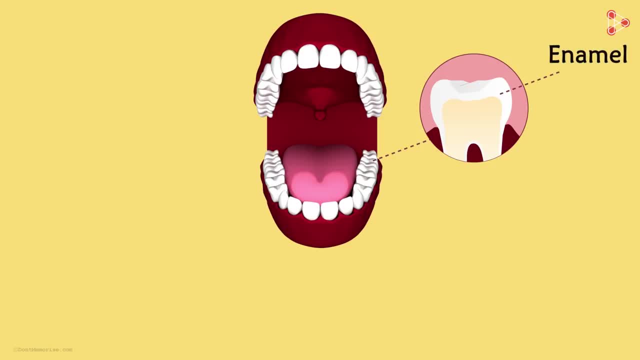 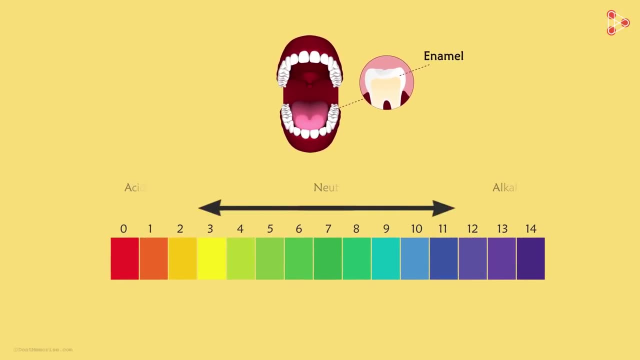 Tooth enamel is the hardest substance in our body and does not dissolve in water and mildly acidic solutions. However, it gets corroded slowly when the pH in the mouth falls below 5.5. But how does the pH fall below 5.5? 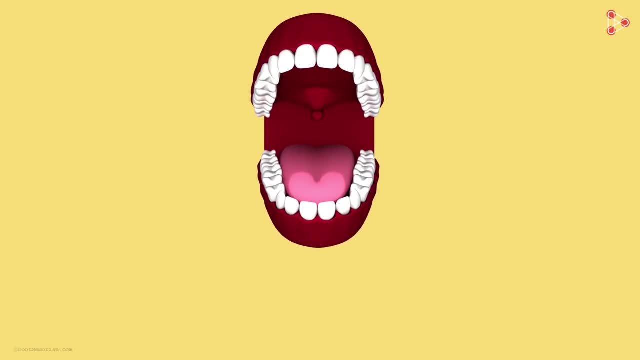 When we eat food, some food particles remain stuck to the teeth. Bacteria present in the mouth produce acid by the degradation of the sugar and fat. The food particles present in the mouth. This is what causes decaying of the teeth. 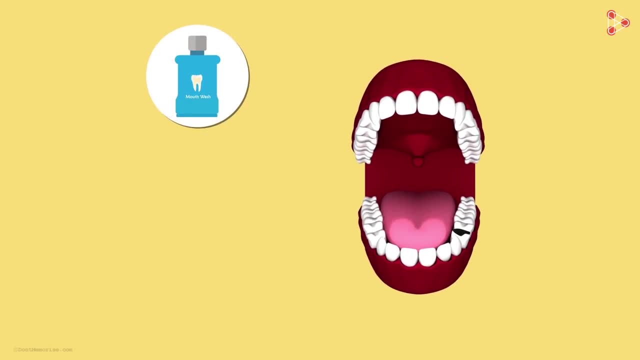 What's the best way to avoid this? We should clean our mouth after eating food. And something even better would be to avoid eating sugary foods. 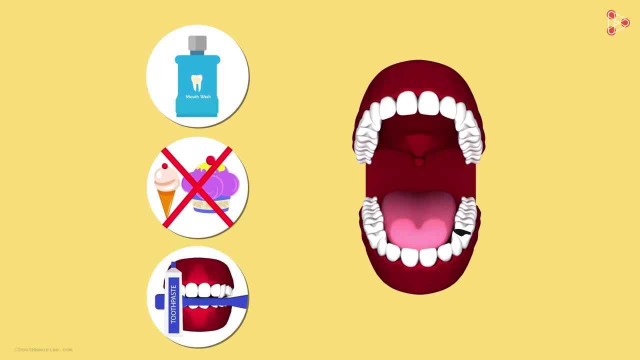 Cleaning the teeth using toothpastes help in preventing tooth decay. 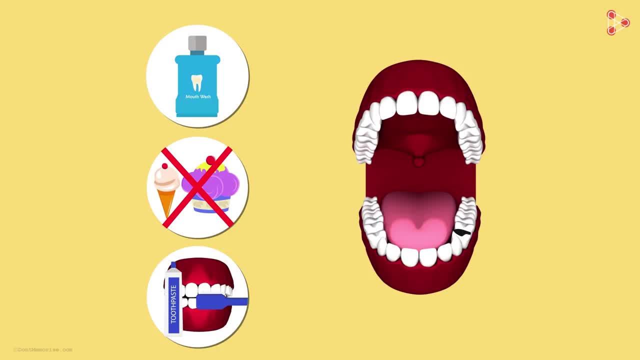 Toothpastes are generally basic and hence they neutralize the excess acid in the mouth and prevent tooth decay. The concept of pH is very simple. Toothpaste is the most important substance in the mouth. 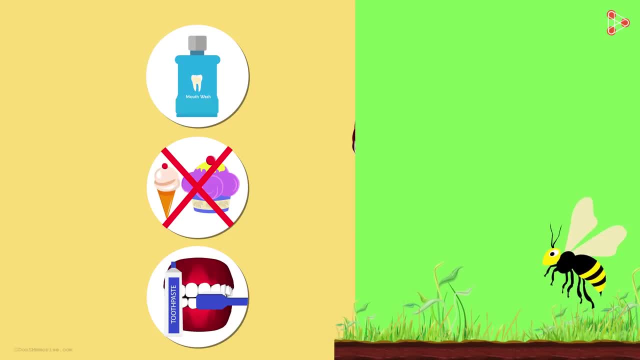 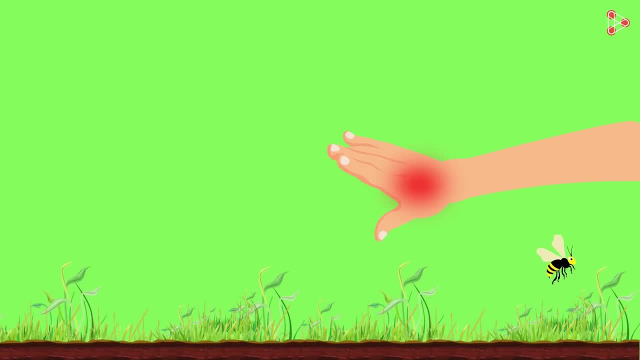 The pH also helps in understanding the self-defense used by certain animals and plants. If you've ever been stung by a honey bee, do you know what really caused that acute pain? 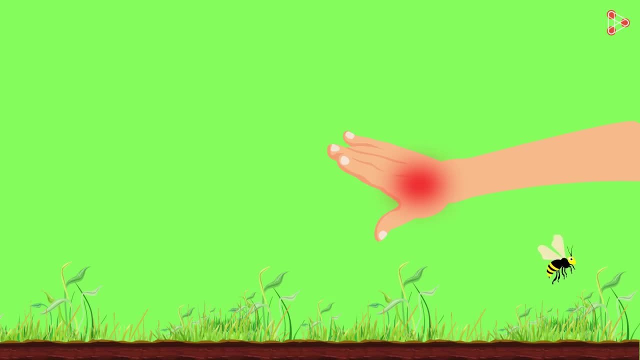 Yes, it's the acid in that sting which caused the pain. So if we use a mild base like baking soda around the stung area, it gives us some relief. 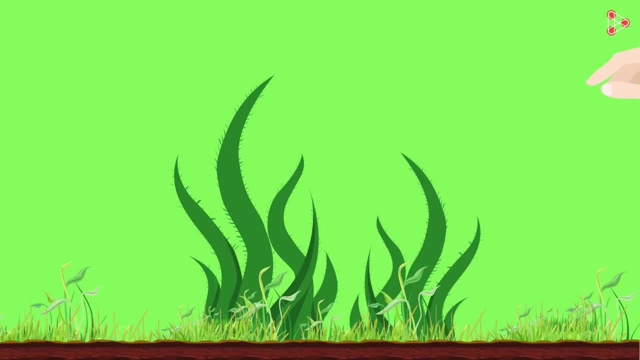 And in nature, there are leaves which have stinging hair and they inject acid upon the stung area. 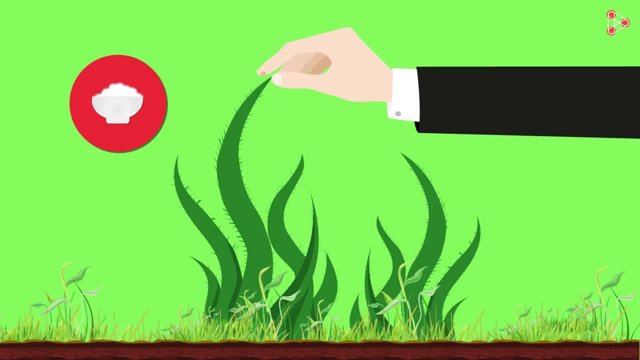 Again, we use something which is basic in nature to get some relief. 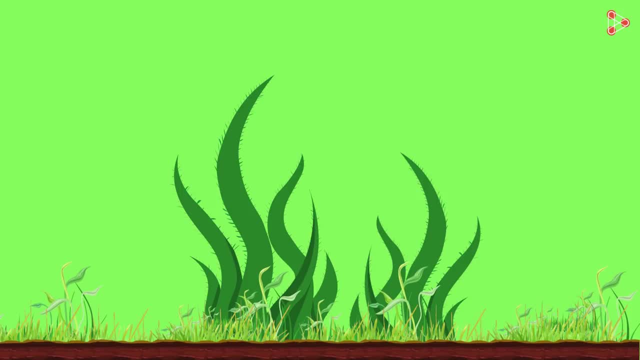 So these were some of the ways in which the concept of pH is used in daily life. 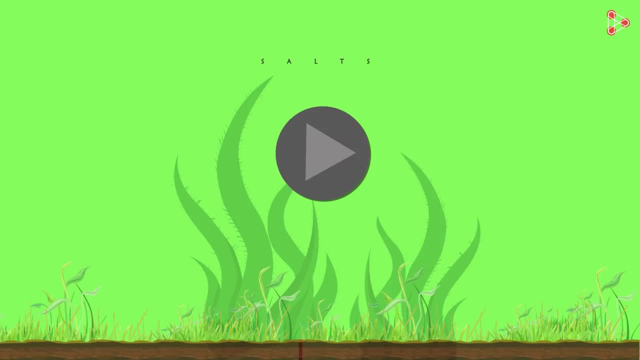 In the coming videos, we will understand more about salts. 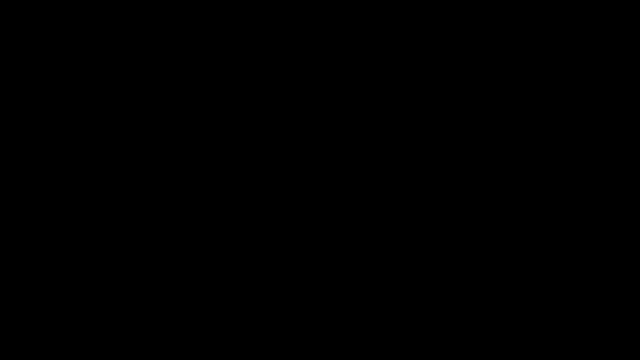 In this lesson, we're going to talk about solving quadratic equations by factoring. 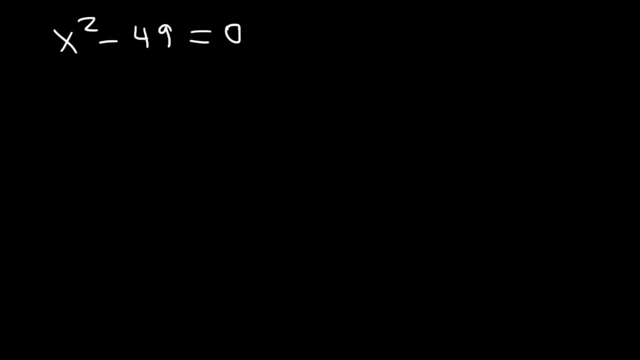 So let's start with this example, x squared minus 49 is equal to 0. You can use the difference of perfect squares technique for this one. The square root of x squared is x, the square root of 49 is 7. So it's going to be x plus 7 and x minus 7. Now you need to set each factor equal to 0 at this point. And then you can find the value of x. So we have x plus 7 is equal to 0 and x minus 7 is equal to 0. The reason why we can do that is because if one of these terms is equal to 0, then everything is 0. 0 times anything is 0. So x is equal to negative 7. 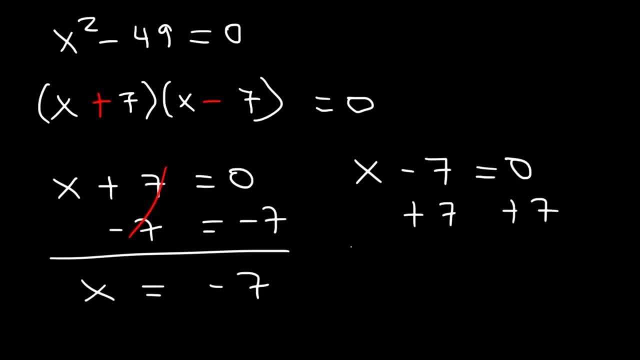 And in the other equation, if we add 7 to both sides, we can see that x is equal to 0. So x is equal to positive 7. 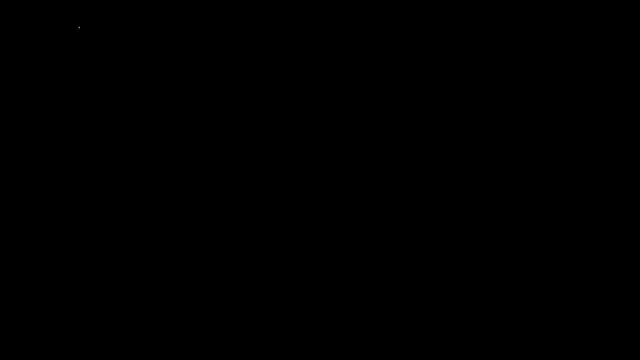 Let's try another example. Let's say if we have 3x squared minus 75 is equal to 0. What is the value of x?